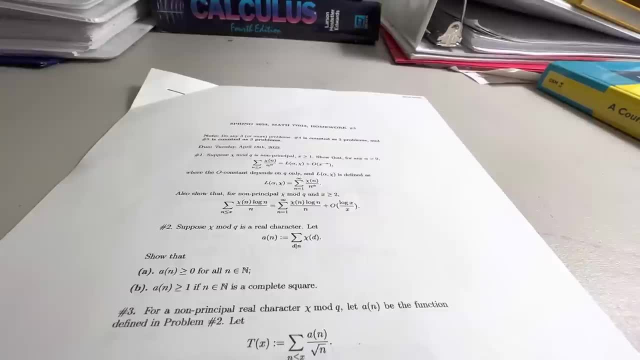 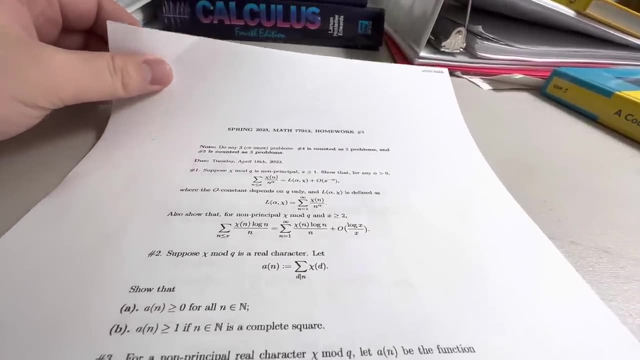 Although, to be fair, I'll probably just follow the instructions and try and get it answered That way Anyway. so I thought I would just make a video about analytic number theory, because I don't talk about the class much. So we'll look at these problems. Here's the first. 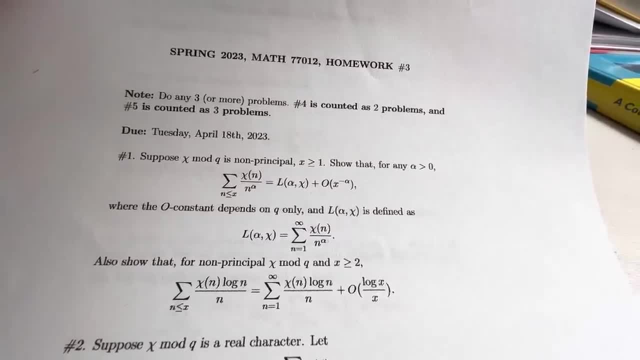 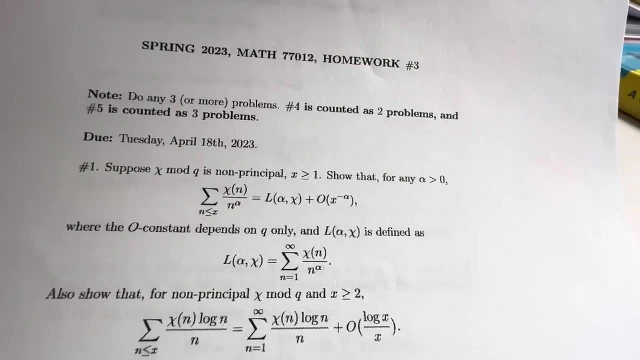 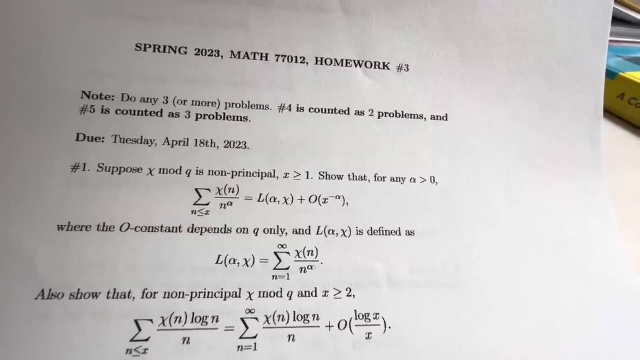 one. Let chi mod q be non-principle, x is bigger than or equal to one. Show that for any alpha positive you have that the sum is equal to the L function alpha, chi plus big O of x. to the negative alpha where the big O constant depends on q only. 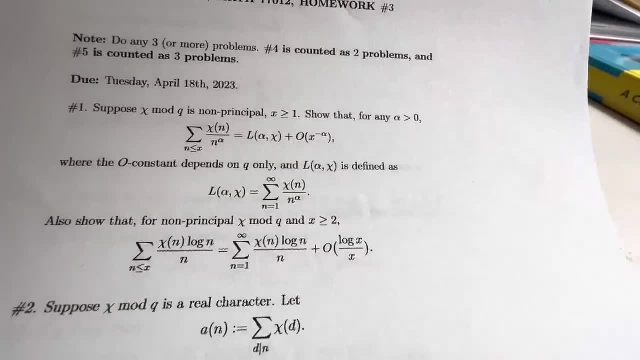 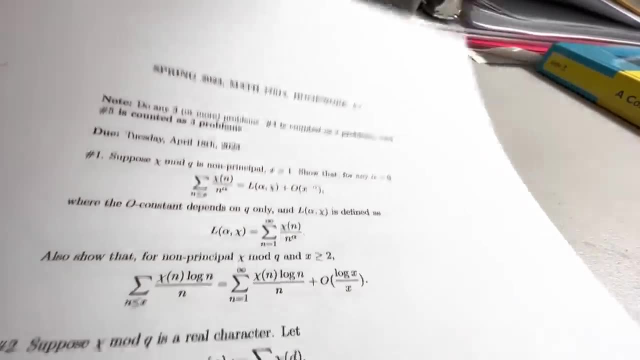 And the L function is defined as follows: Also show that for non-principle chi mod q, x bigger than or equal to two. you have this equation here, So I looked through this homework assignment before recording. I think number one's not too bad. 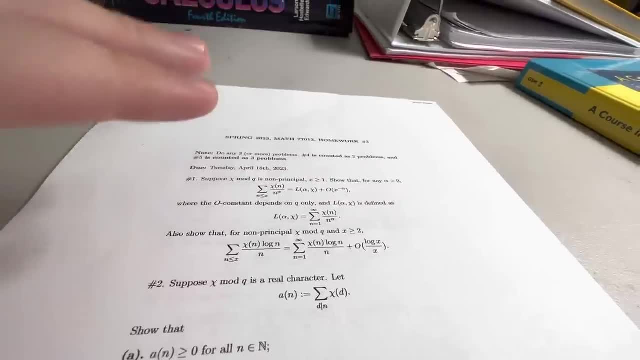 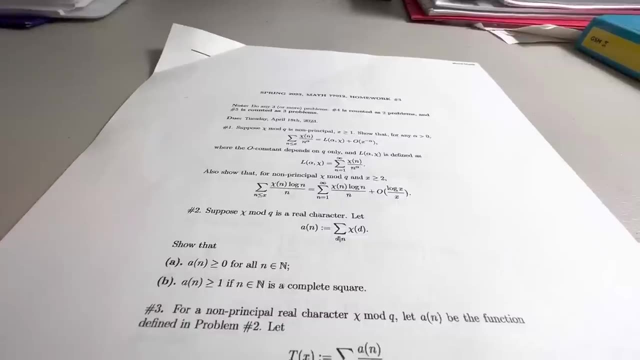 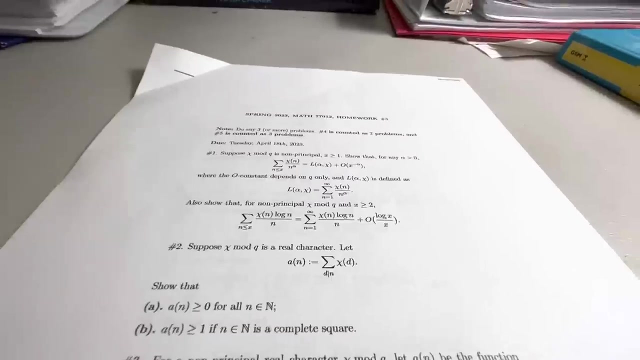 His homework assignments are usually very much like. if you understand the notes or if you look at the notes for inspiration, then the homework problems aren't too bad. Other classes that I have the homework or, excuse me, the notes don't really help too much with the homework, But for this guy. 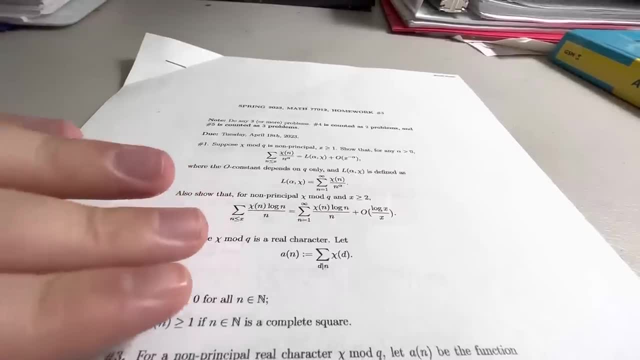 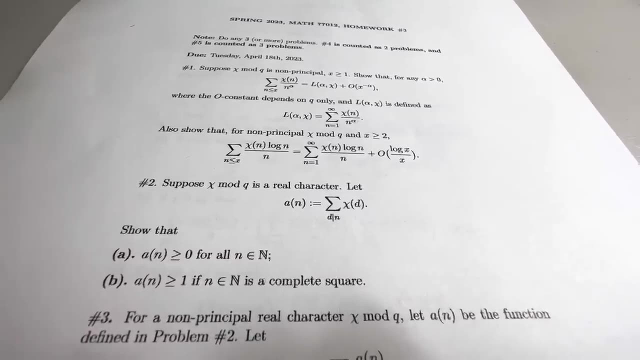 that doesn't seem to be the case. As long as you have the notes in front of you, you can piece together an argument that makes a lot of sense. Okay, so suppose chi mod q is a real character. Let a and b defined as follows: 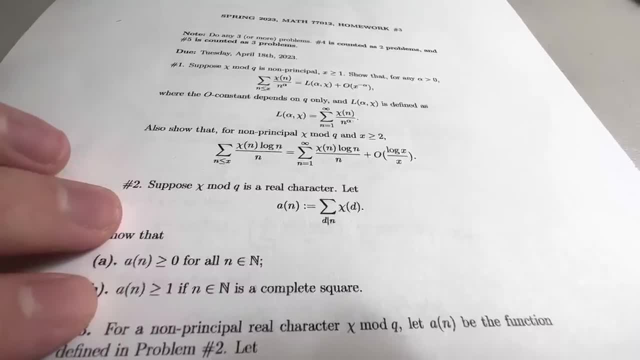 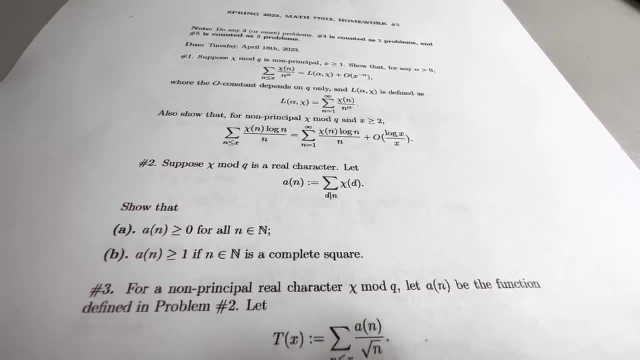 Show that a and non-negative for all n integers and prove that a and bigger than or equal to one is a complete square. That one might not be too bad either. I have to look over my notes. It's been a while since I've read through it. 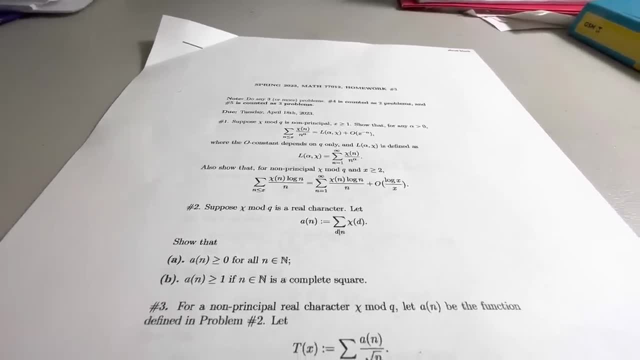 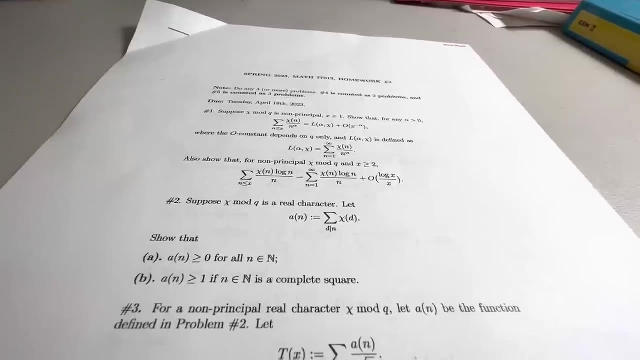 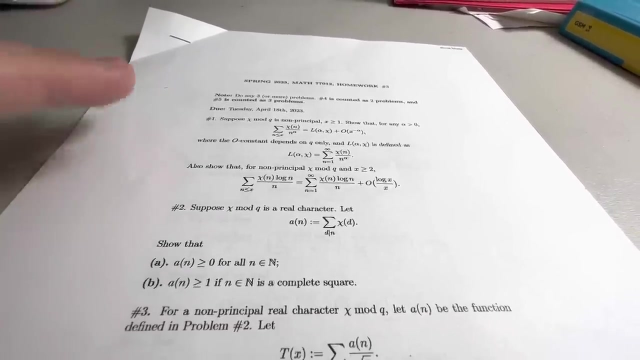 The problem with this is that my probability theory exam- the second one- is in like two weeks and I haven't really studied for it because I was stupid and did not study. over the break I studied a little bit, but I studied like in the beginning and then I got caught up doing other things, so I didn't really study. 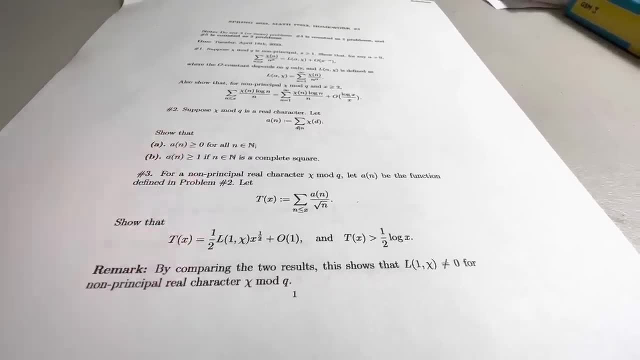 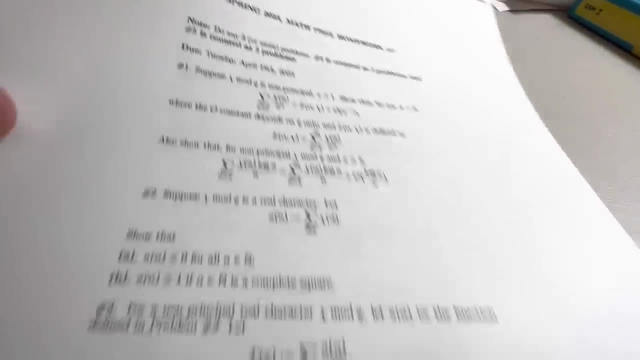 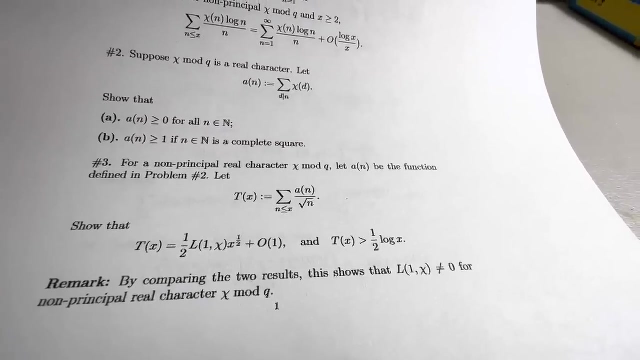 Which means now I have to juggle this assignment with studying for that probability test. You can see up here that the assignment is due April the 18th, so I have a couple days to do it. For non-principle real character, chi mod q, let a and b a function defined in problem two. 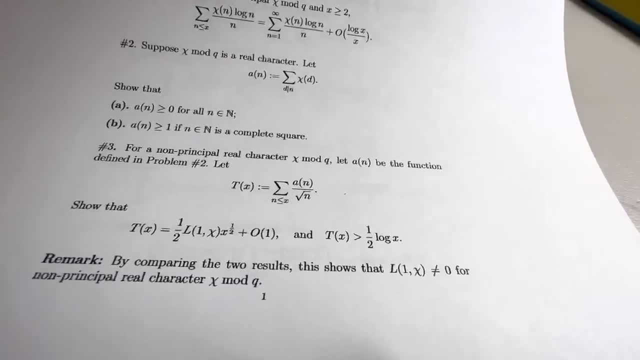 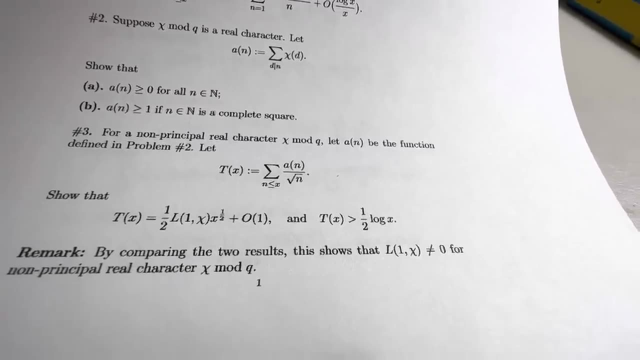 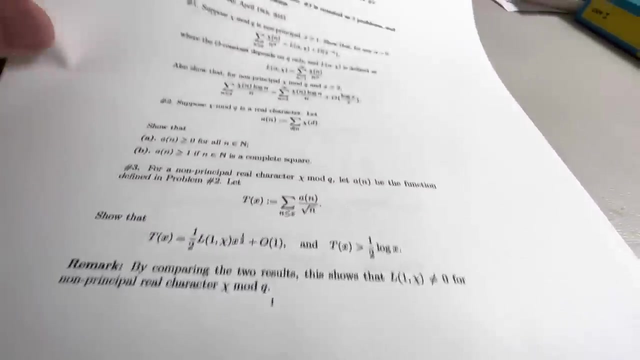 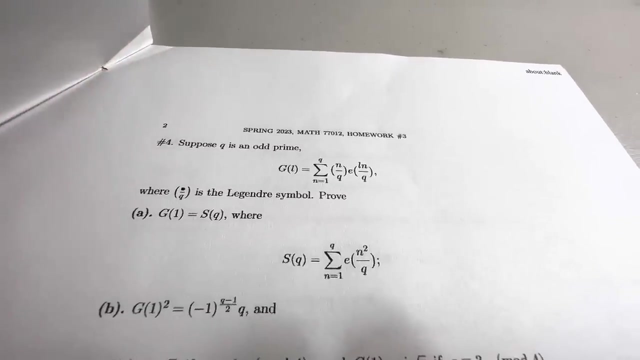 Let tx be defined as follows: Show that tx is equal to one-half l, function one chi x to the one-half plus big O, And that tx is bigger than one-half log x. And then he has a remark: Okay, problem four, I believe problem four, he said, would count it as two problems. 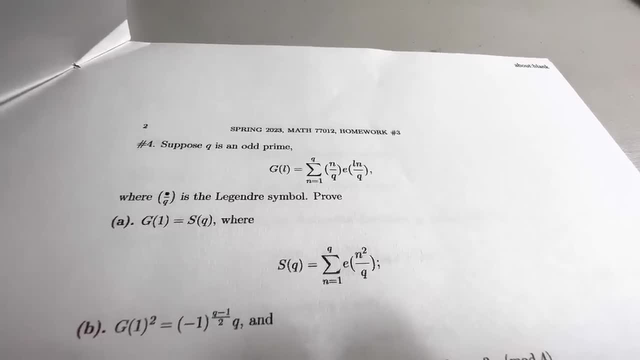 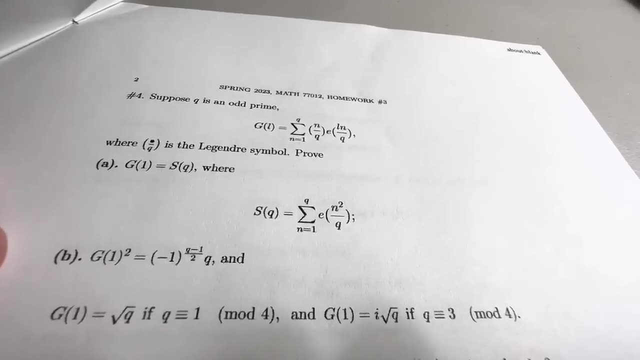 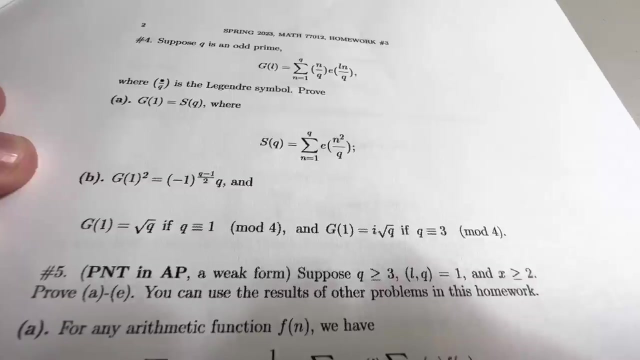 Suppose q is an odd prime. gl is defined as follows: a genre symbol and we want to prove that g1 is equal to sq or, yeah, g1, where sq is equal to this guy, Prove that g1 squared is equal to negative, one raised to the q minus one over two q. 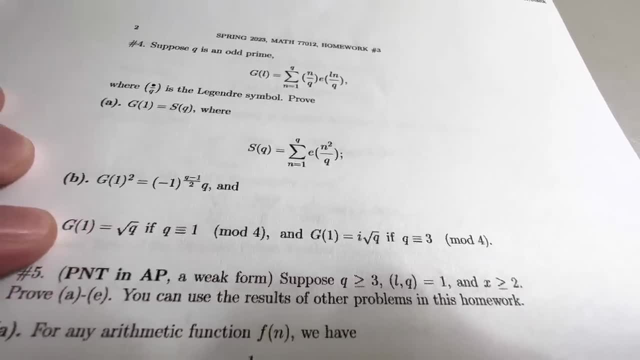 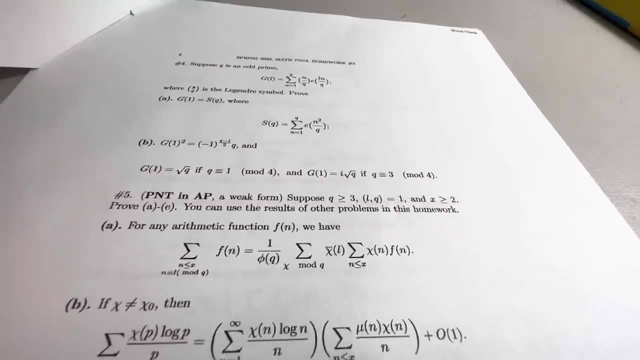 and this equation. I'm not really a big fan of number theory. There are, I'll put it this way, there are topics in number theory that I like, like the Riemann state of function, but as a whole I'm not a big fan of number theory. 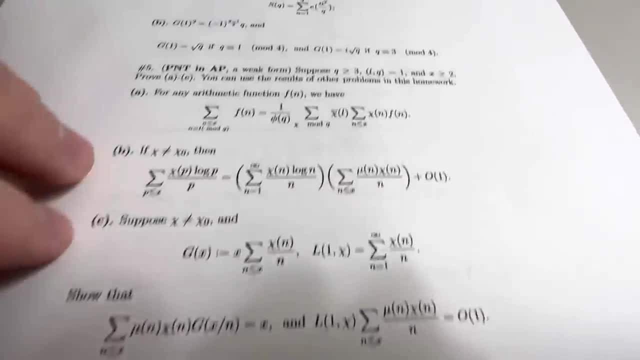 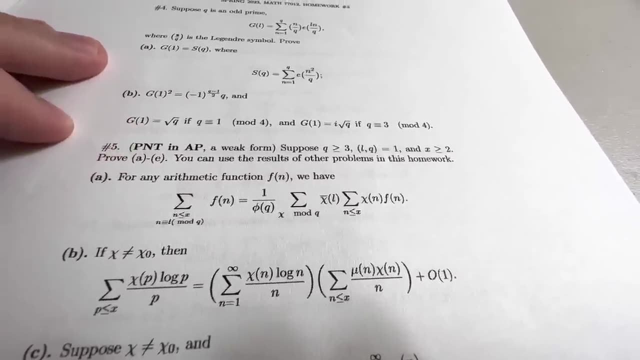 Okay, number five. So number five is the one where if you solve number five, you don't have to do any other problems. And it's about the prime number theorem. So p and t stands for prime number theorem. I'm not sure what a p stands for here. 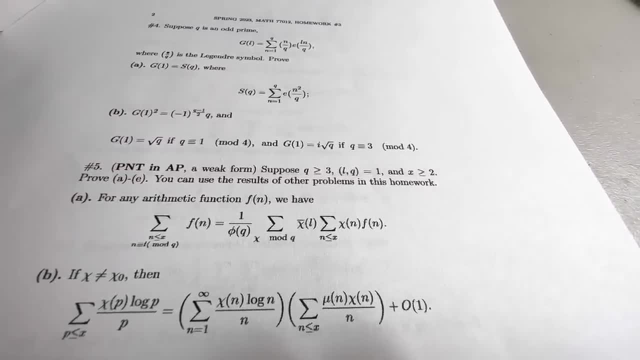 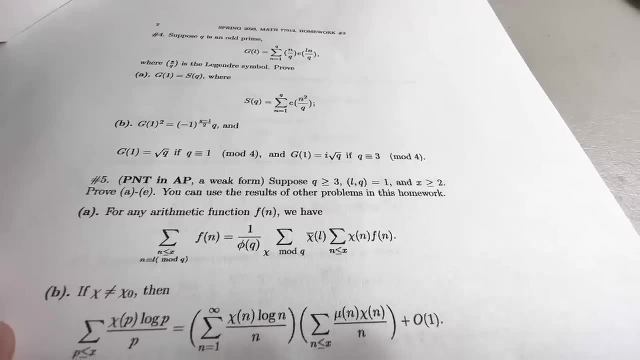 Suppose q is bigger than equal to three, the gcd of l and q is one, so they're co-prime, and x is greater than equal to two. Prove a through e. You can use the results from other problems in this homework. 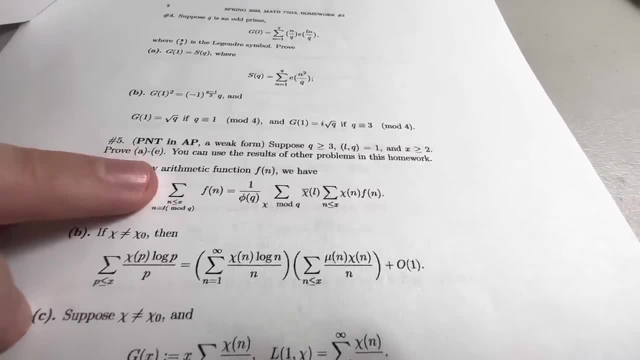 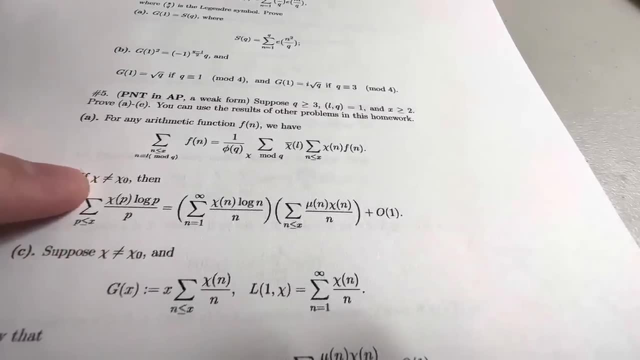 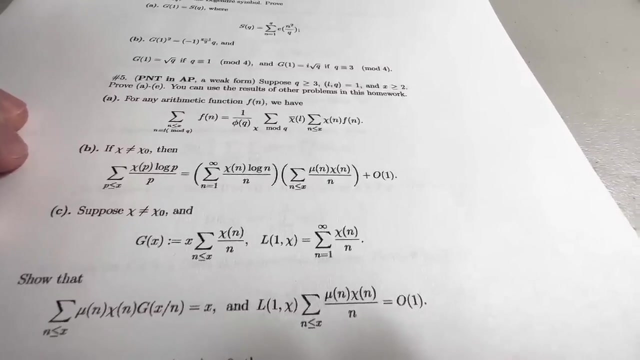 For any arithmetic function, fn. we have this equation, So we have to prove that If chi is not equal to chi zero, then this sum is equal to this thing. Suppose chi is not equal to chi zero and gx is this, and now one, chi is that. 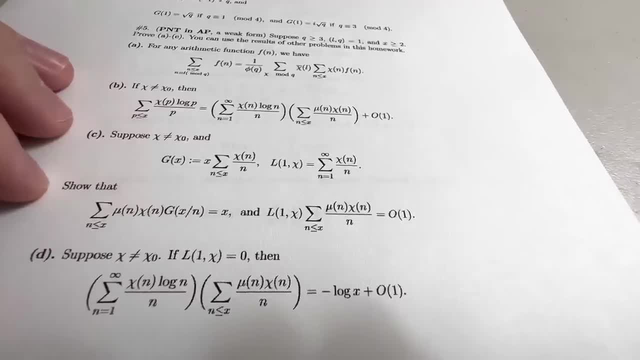 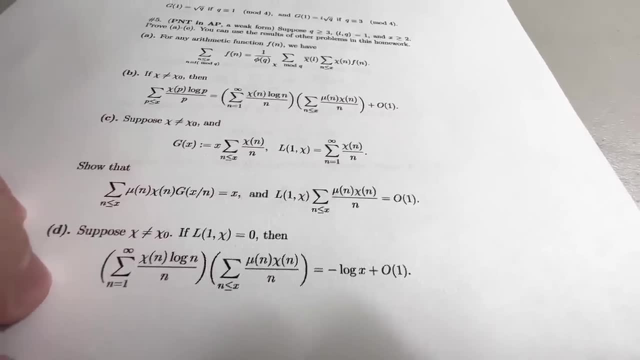 Show that we have this relation, or two relations that are. that is Man. this doesn't look easy, does it? There's a lot of symbols here. If you don't know what the symbols mean, you're kind of stuck. 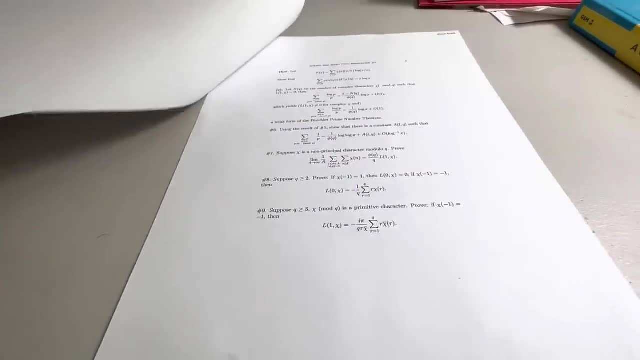 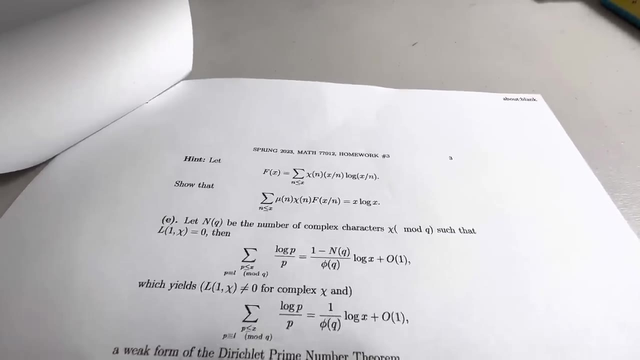 But if you know what the knowing the definitions is half the battle in a lot of these graduate courses. As long as you understand what the symbols are, the work is half done. You just have to use some tricks you pick up along the way in class. 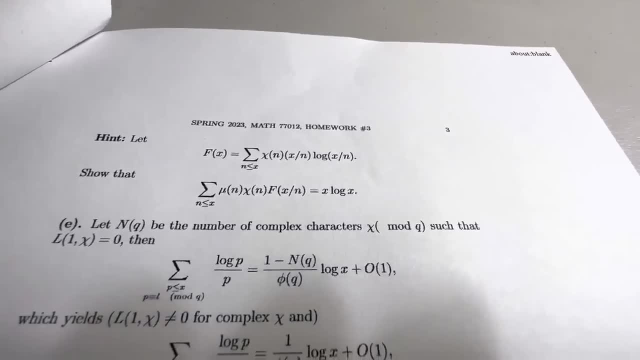 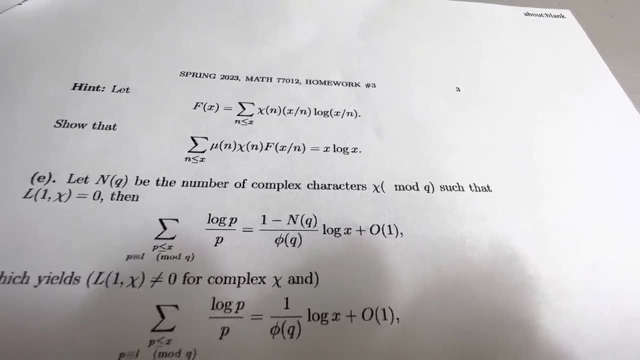 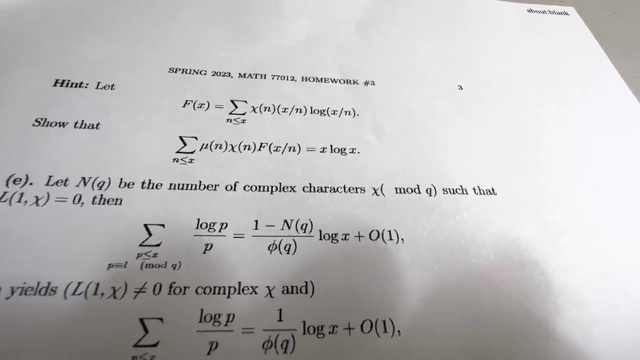 And he gives us a hint which is kind of nice. Part e: Let nq be the number of complex characters, chi mod q, such that l1 chi is equal to zero. Prove that this sum of log p over p is equal to one minus nq over phi q. log x plus big O of one. 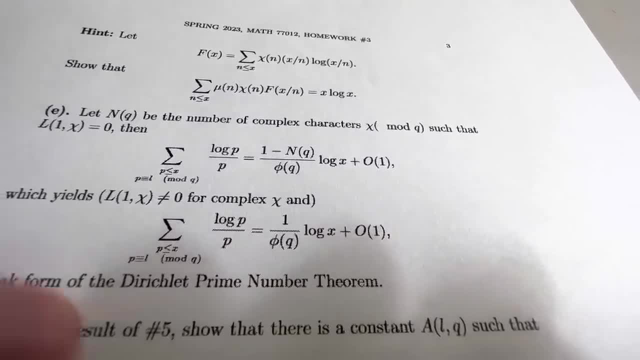 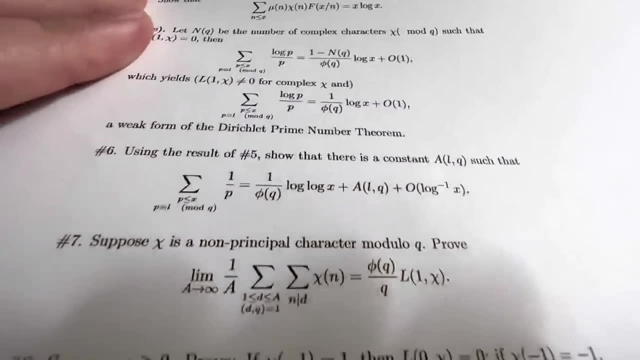 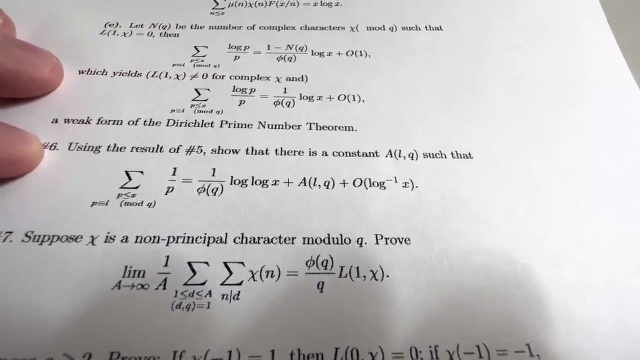 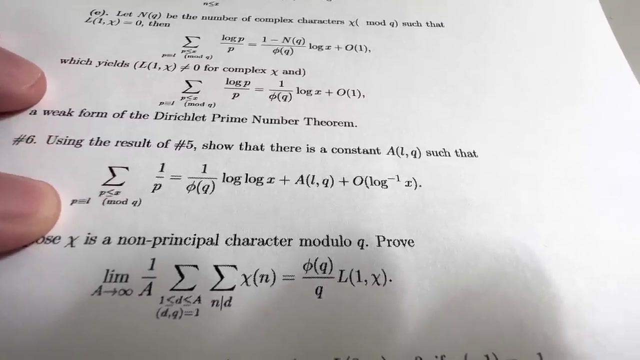 Which yields this thing. Number five, Using the result of number five or, excuse me, number six, Using the result of five, show that there is a constant a, l, q, Such that this sum of one over p, where p is congruent to l mod q. 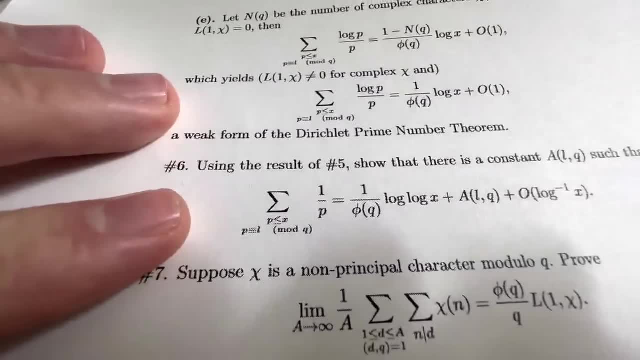 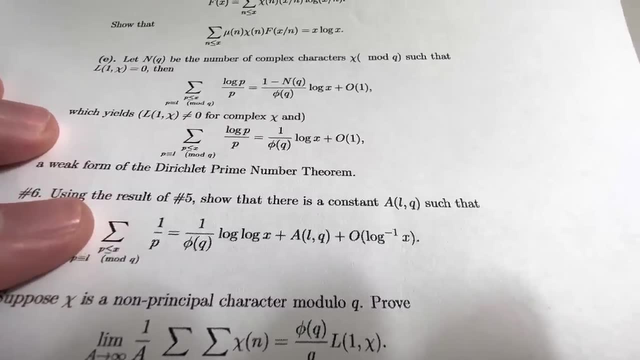 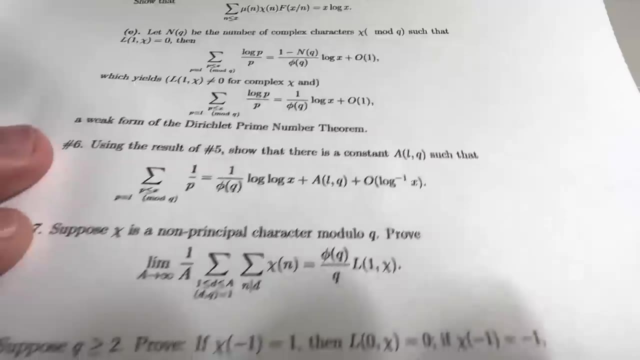 Is that an l or a one? I can't read it. I think it's an l Anyway. so the sum is equal to one over phi q log log x plus a l q plus big O of log inverse of x Oh number theory. 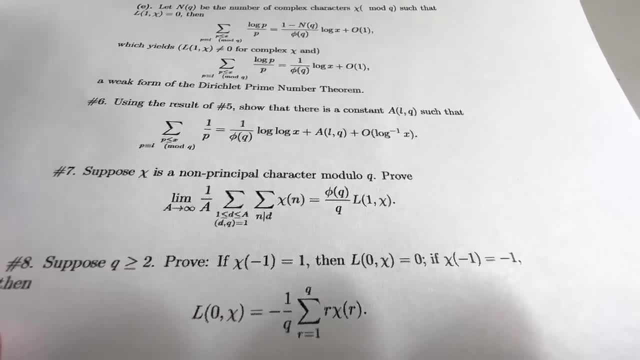 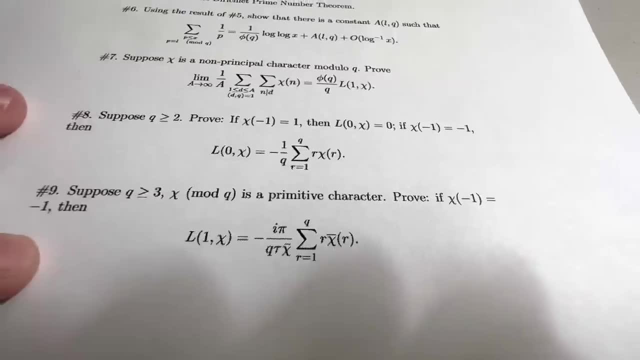 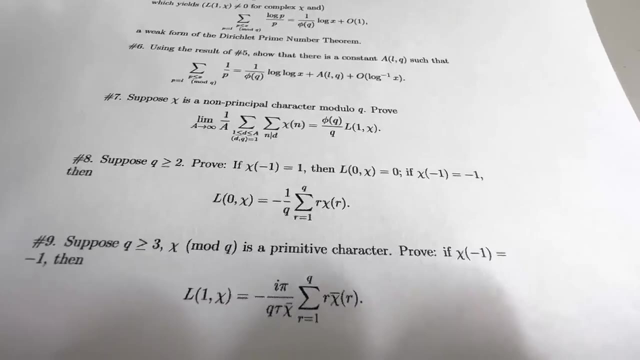 Suppose chi is non-principle character Modulo of q. prove the following: I can already tell you that I'm going to have to search the internet for some of these solutions. My number theory is not that great. Suppose q is bigger than equal to two, Prove the following: 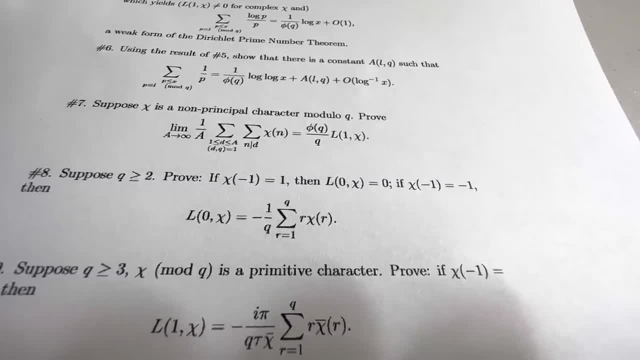 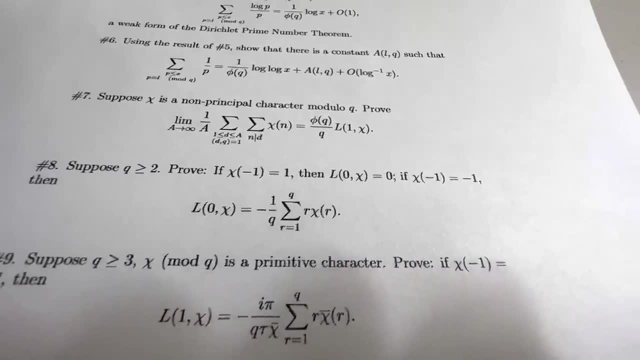 Chi of negative one is one, then l0 chi is zero. If chi negative one is negative one, then l0 chi is equal to this expression. So this is the number theory that we are doing to solve this problem. So it looks to me, just by looking at these problems, that I need to review my characters. 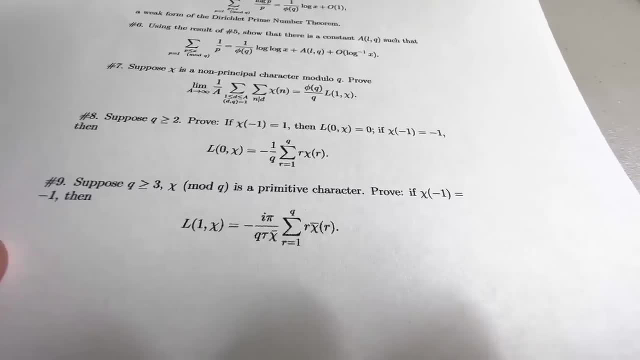 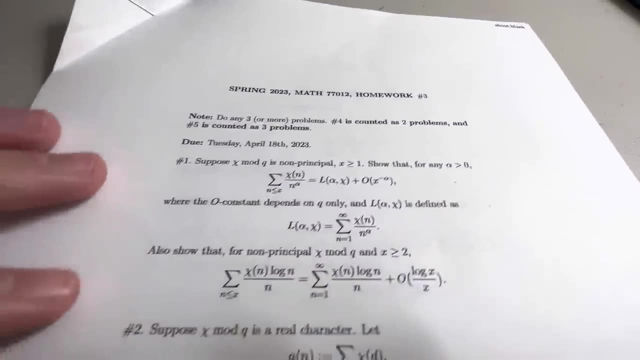 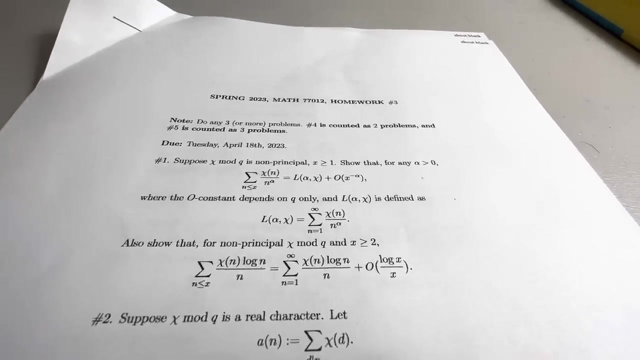 They're not the characteristic functions here. They mean other things. but I did not take algebraic number theory. I just went straight to analytic number theory. I kind of wanted to take algebraic number theory last semester, but there's, I need to review this. 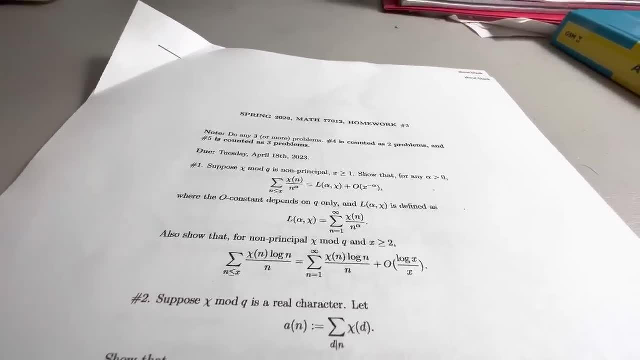 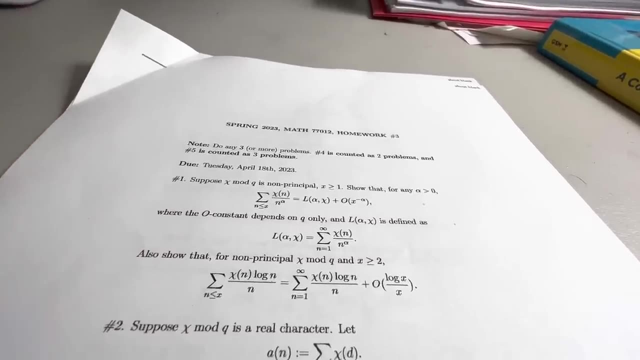 Let me just see. Okay, There's no way I would have been able to take it Probability Theory 1, and then the Potential Theory that I took as well as Complex Variables 2, because I took Complex Variables 2 last semester. 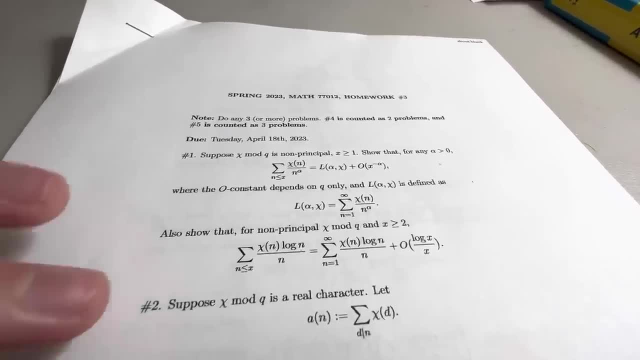 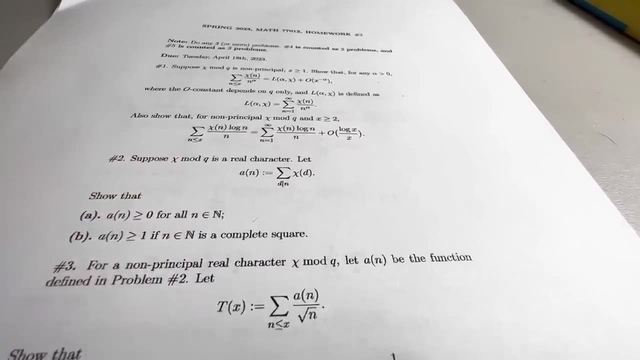 There have been four classes. There's no way I would have been able to do that, plus teaching on top of that. But so far from the other people that are in this class that did take Algebraic Number Theory. they said that this is very different from last semester. 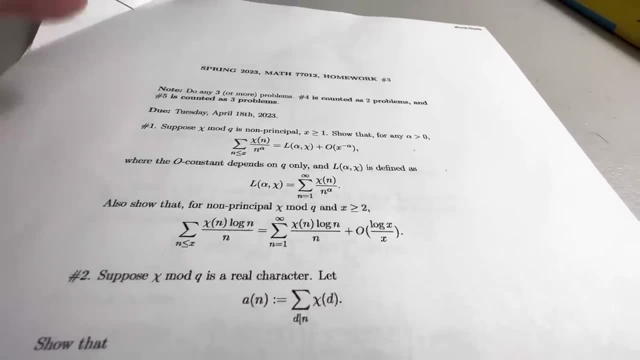 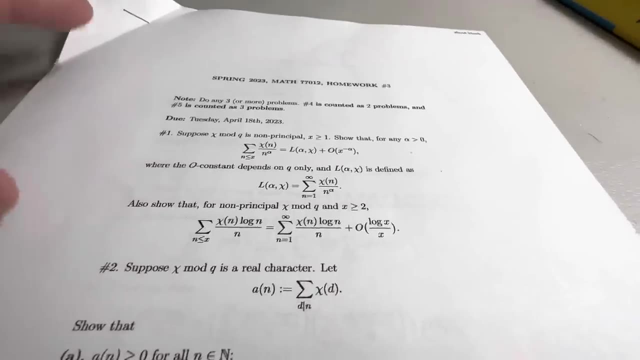 But it would have been nice to have a complete rounded. what do you say? course selection? I don't know what I'm trying to say. It's too early in the morning for me and I need to get ready for work. 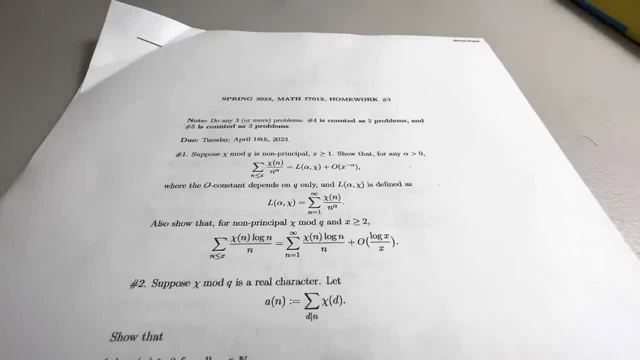 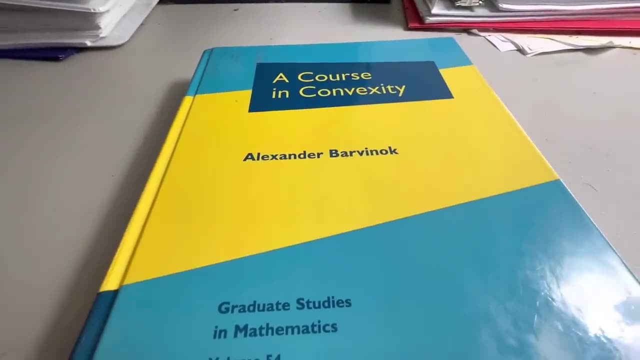 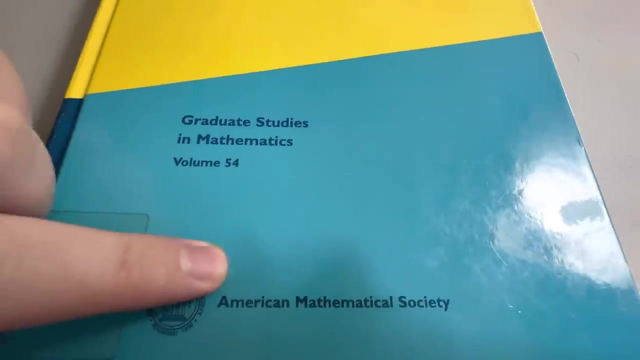 So this morning I'm actually going in to take my Convex Geometry class and I actually got a book in Convex Geometry which is over here Course in Convexity. It's an AMS book, so whenever you see books that have this cover, it's usually from the American Mathematical Society. 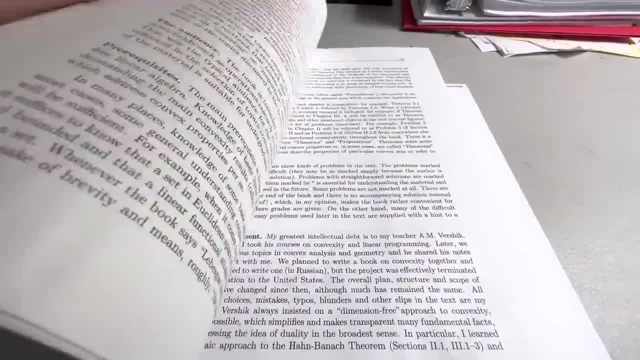 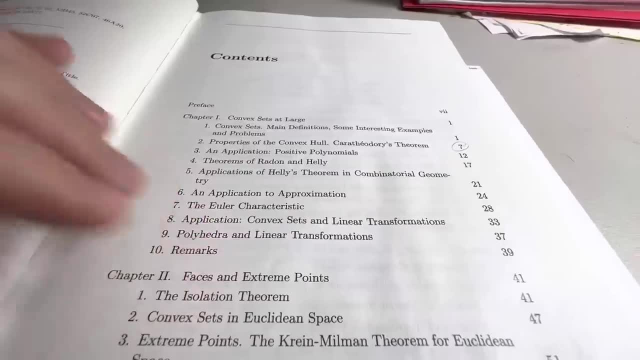 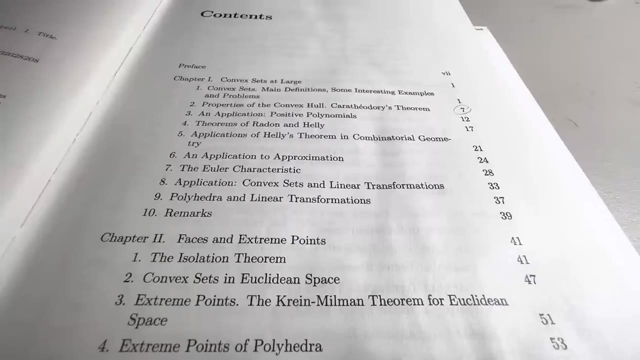 These AMS books are really good so far. I went to the library at my university and my library is pretty huge, but I did not expect them to have as many textbooks on mathematics as they did, because I went to their section to look for a very specific math book, which I'm going to make a video over here shortly. 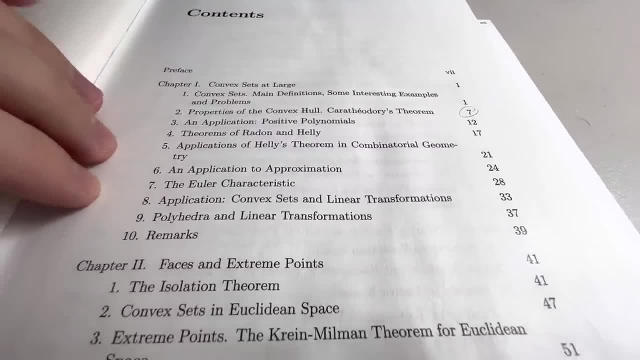 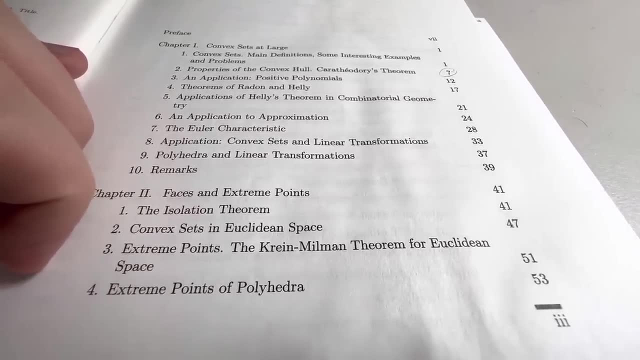 But when I was there I found it. but I also just looked at all of the books that they had and I was a bit surprised And I wanted to check out a bunch of them. but there's no way I would have been able to read all of the books I wanted to read. 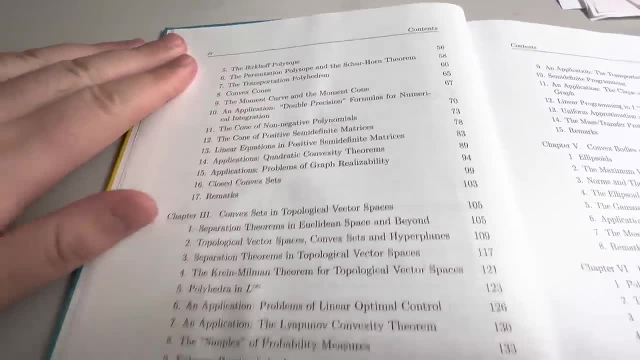 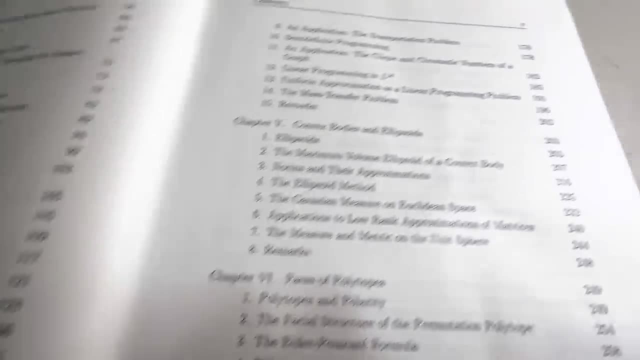 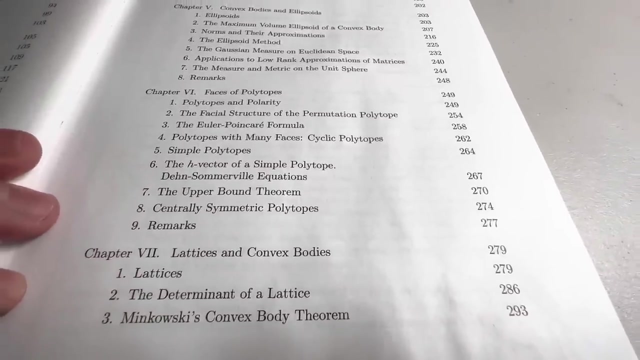 But I found this book and I thought that it was too good to pass up, so I decided to borrow it and at least read through it. I'm still working on chapter one. I just borrowed it yesterday, But I think it might help me in my research because my geometry background is a bit limited. 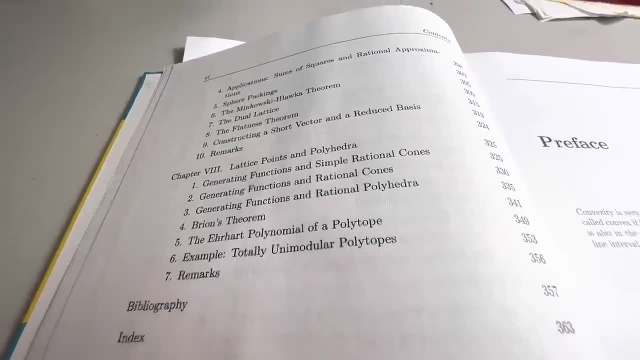 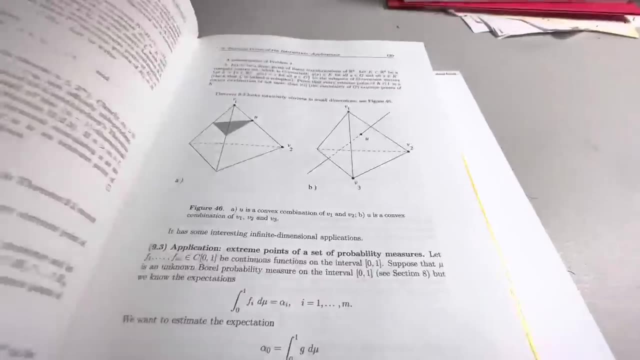 Hold my camera steady so you can read the table of contents, Because I looked up the table of contents just to flip through it and then I read just a tiny bit, Like I opened up somewhere random in here and just looked at the way it was formatted. 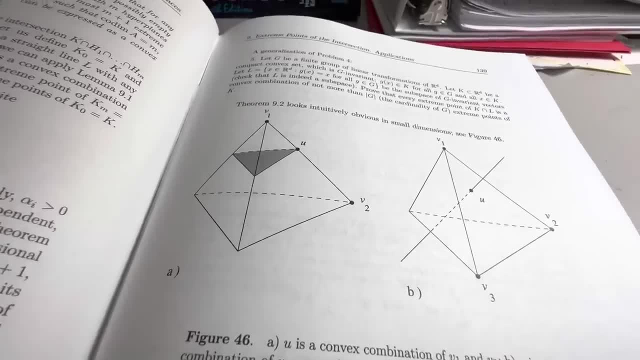 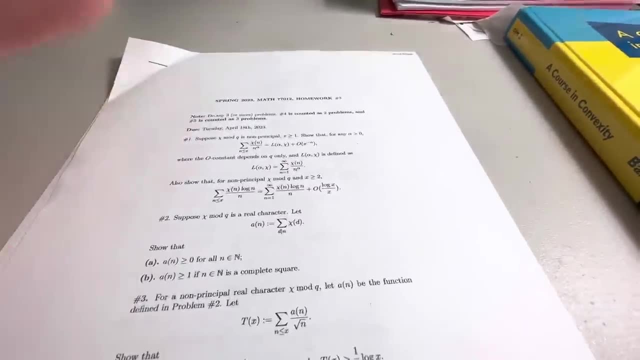 And I was like, okay, Maybe I should consider checking this book out and reading it. Hopefully it'll be worthwhile Anyway. so that's what's on my to-do list. This guy study for probability theory and then casually read my convex geometry book.